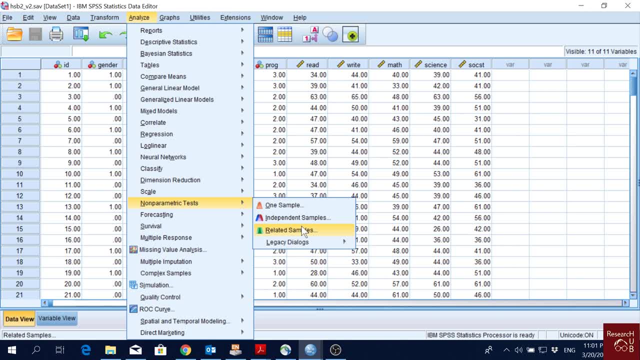 when we have multiple times data collected repeatedly in multiple times, then we'll go for repeated samples. okay, so that's how it is, but actually, interestingly, if you just pick one of them, and if you with this version of spss, if you just pick one of them, i'm using the spss 25 version, so if you just click one of them and put your data, it 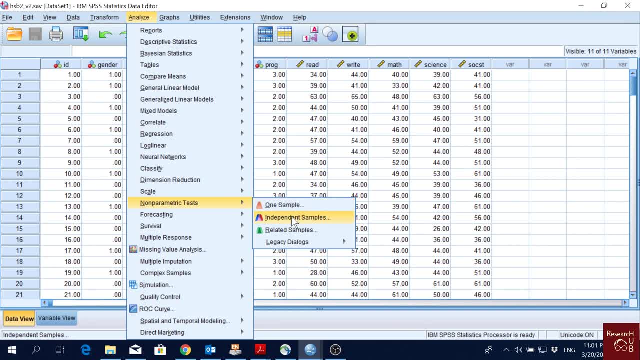 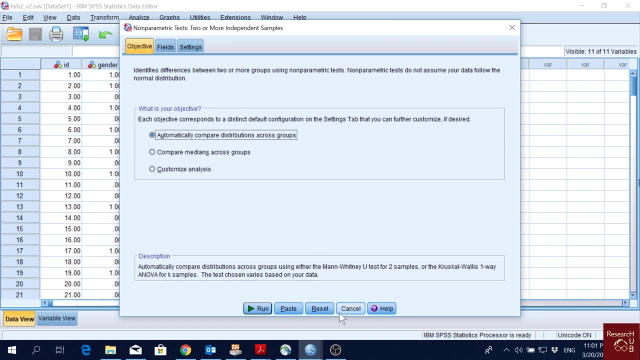 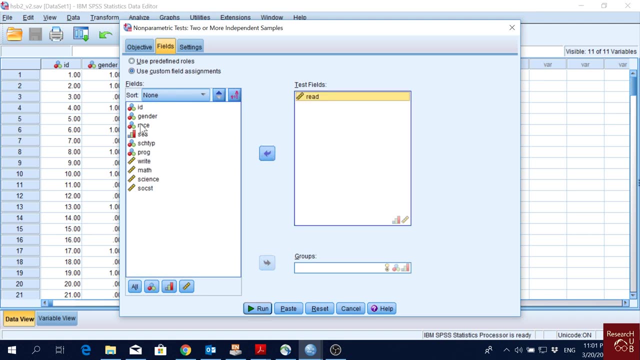 will choose the appropriate test automatically. so let's see. let's see, i'm picking independent samples here. so automatically compare distribution across scripts. okay, and i'll go to field. i will put my data here. so let's say, i want to pick three categories, so i'll just put the group here, okay. so if you want to compare with two, 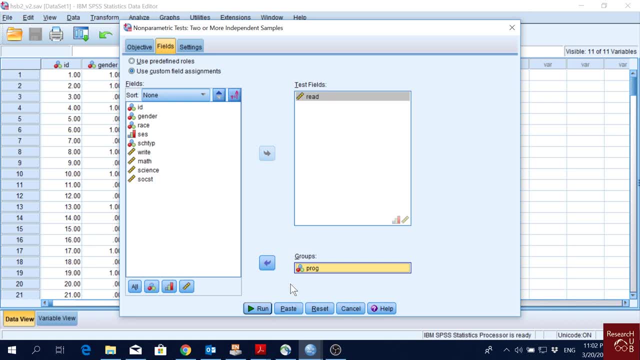 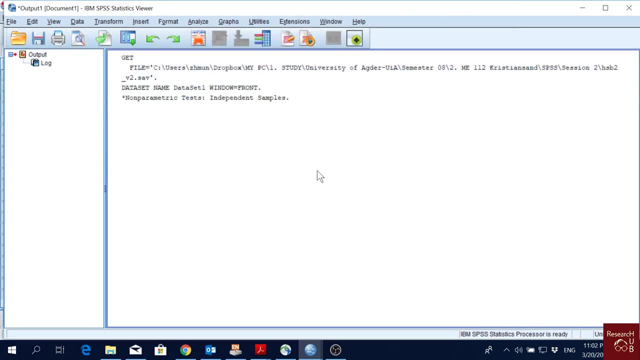 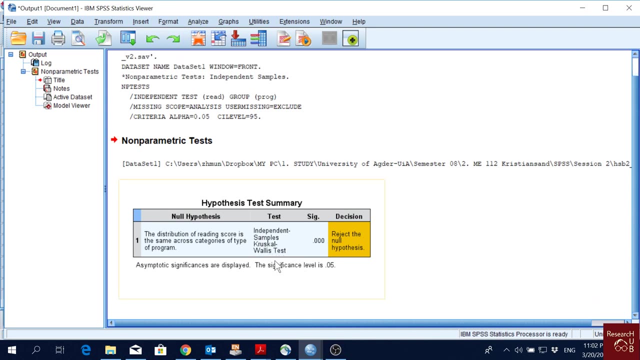 groups. just put the two group variable here, so whatever you want. so i'm putting three groups here, okay, and i'll click run and you'll see it will pick. yeah, it picked. independent samples. cruise call wallace test. okay, this is the appropriate test when we have more than two categories and data is non-parametric. 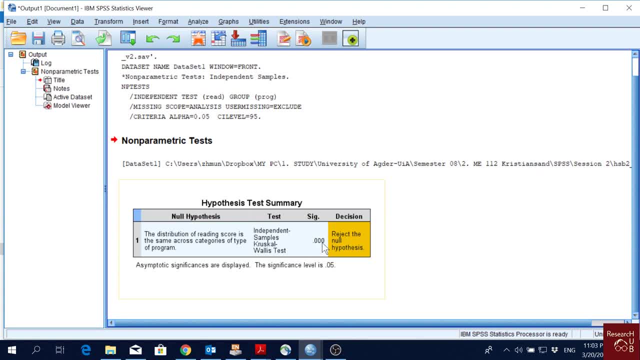 and here you see, the significance value is zero, zero, zero, zero, and we reject the null hypothesis which is also given here. the distribution of the reading score is the same across categories of type of program, so we reject it. that means there is a significant difference across group for the reading score. okay, so that's how we can do non-parametric test. 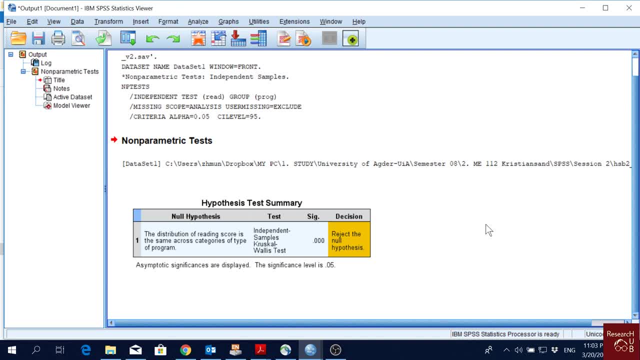 so if you like the video, please comment, share, like and subscribe to our youtube channel.